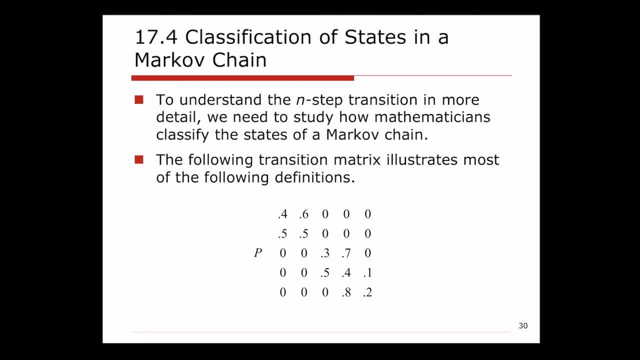 100-step transition probability matrix. 200-step transition probability matrix. What if n or number of steps goes to infinity? in that scenario, how the Markov chain will behave? And to be able to get to that discussion, I need to introduce the different classifications. 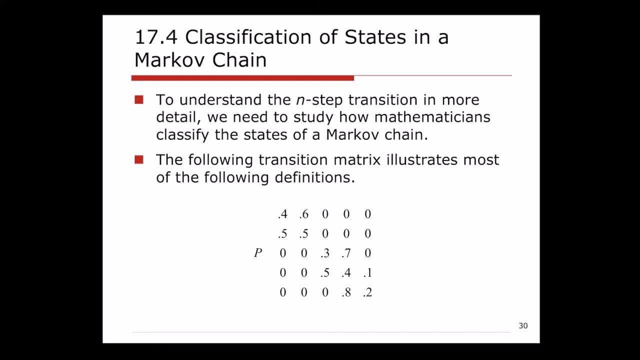 For the states of the Markov chain, because we are going to use this concept. So to be able to do that, I'm going to use these metrics, these transition probability metrics, as an example to explain some of the definitions. So here in these metrics, as you can see, I have 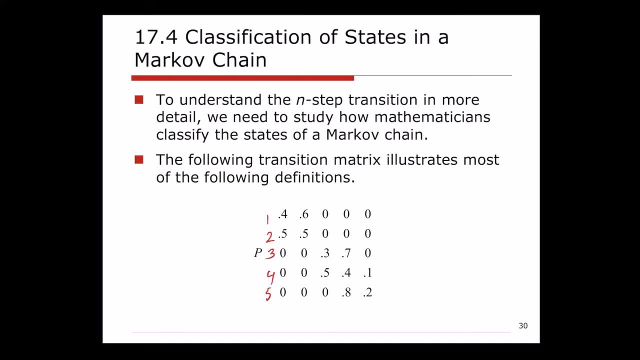 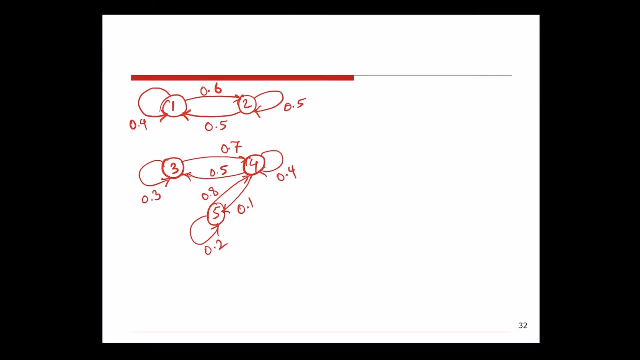 five different states. okay, I'm going to draw the state diagram of these transition probability metrics so that I can explain these definitions or these classifications For you clearly. So this is the state diagram of the transition probability metrics that we just met. So I want you guys to pause the video at this point and draw this state diagram yourself. 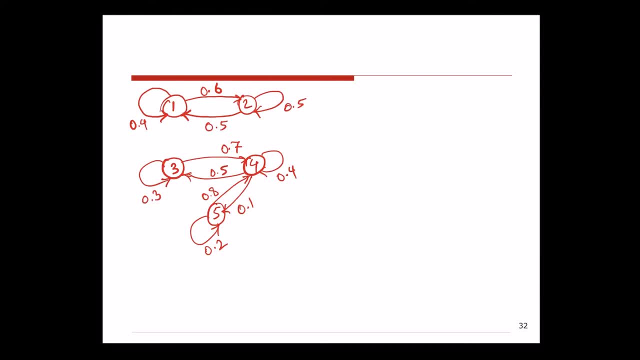 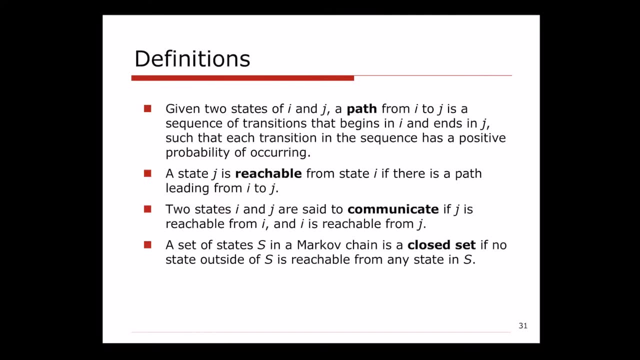 and see if you get similar diagram to the one that I developed. So now let's look at the definitions that we have. So we say that there is a path between state i to j if there are a sequence of transitions that can take us from state i to state j. So we say that there is a path. 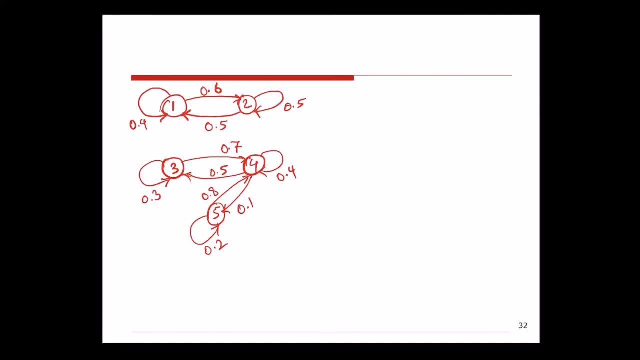 between state i to j, For example. here we say there is a path between state 3 and 5.. Why? Because we can find a sequence of transitions that can take us from state 3 to state 5.. For example, we can go from state 3 to state 4 and then from state 4 to state 5, okay, So there is a sequence. 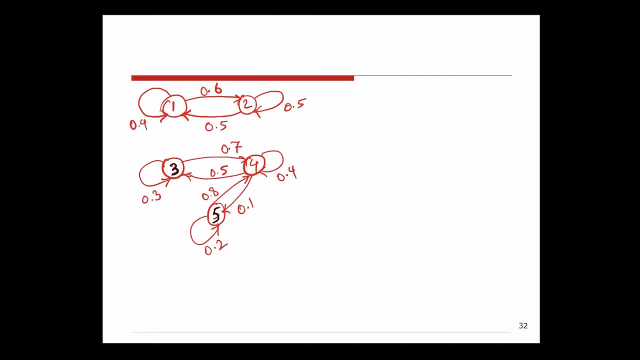 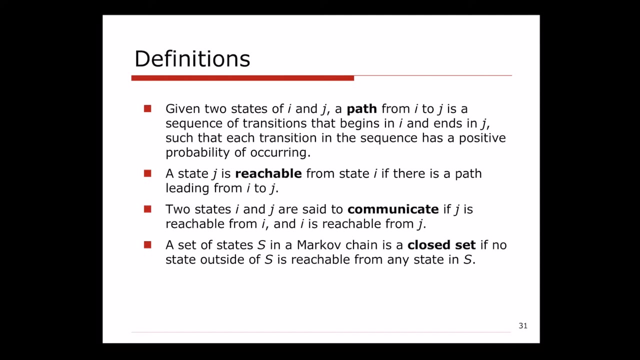 of transitions that can take you from state 3 to state 5.. For example, there is no path between state 1 and state 3 because there is no transition or sequence of transitions that can take us from state 1 to 3.. We say: state j is reachable from i. if there is a path that takes us from i to j. 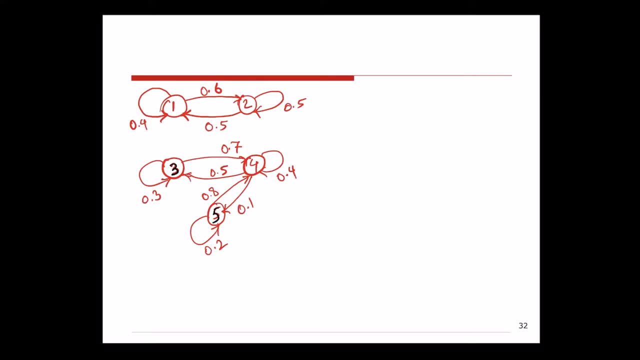 So here, for example, if there is a path that can take us from state 3 to 5, we say that state 5 is reachable from state 3, okay, So so far we covered the definition of path and then definition of reachable. So we say state 5 is reachable from 3 if there is a path that can. 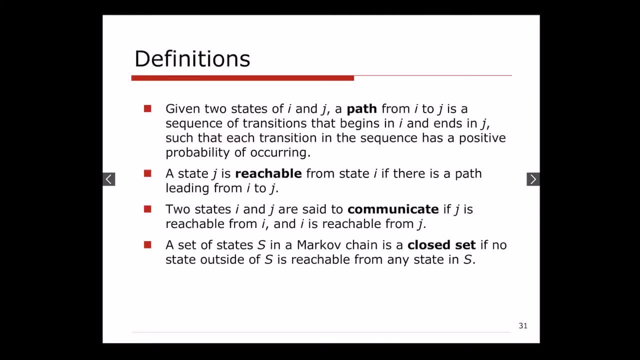 that can take us from 3 to 5.. And then we say two states communicate if there is a, if a state i is reachable from j and state j is reachable from i. So again, if we look at state 3 and 5, for example, 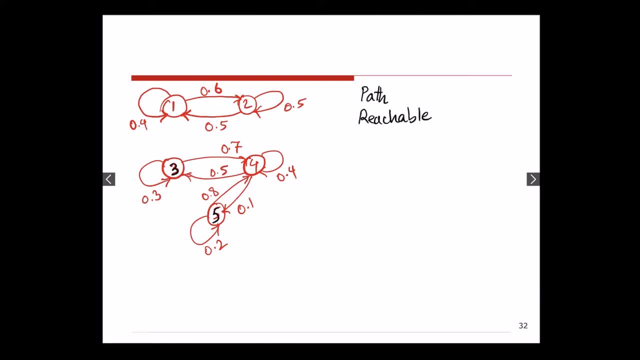 here we have a path from state 3 to 5, which means 5 is reachable from 3.. And we also have a path from state 5 to 3.. We can go from 5 to 4 and then 4 to 3.. There is a sequence of transitions that can 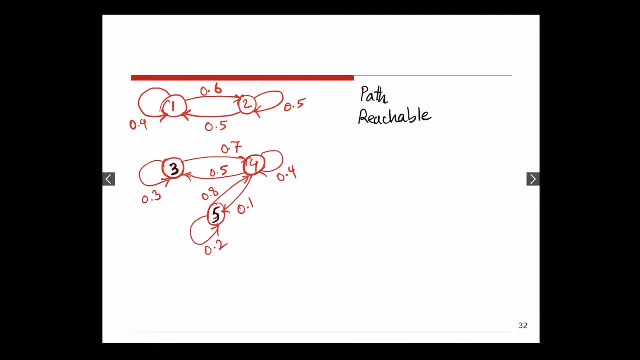 take us from 5 to 3 as well. So state 3 is also reachable from 5.. So so we can say that state 5 is reachable from 3.. State 3 is reachable from 5.. So state 3 and 5 communicate. That's the other. 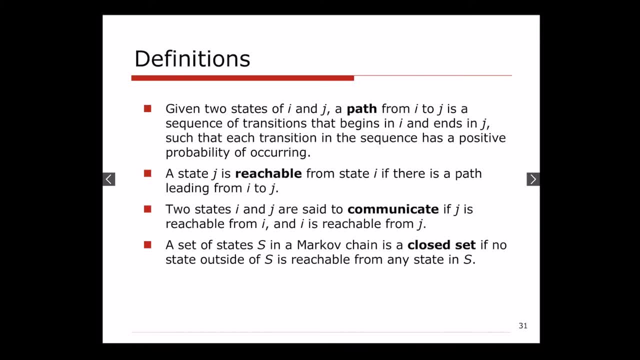 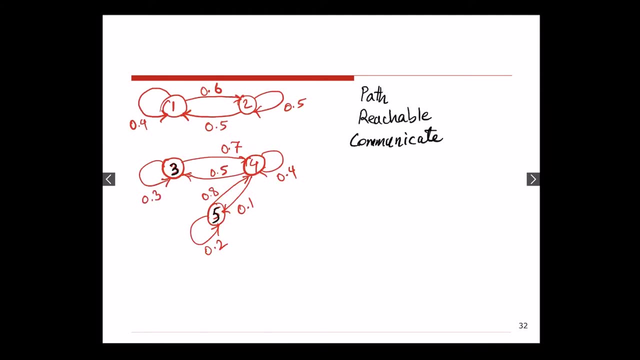 definition we have. And then we have: we have a closed set of the states if that set of states is not reachable from any other state in the, in the samples, in the state space. Okay, So for example, here we say that state 1 and 2 form a closed set, States 3,, 4,, 5,. 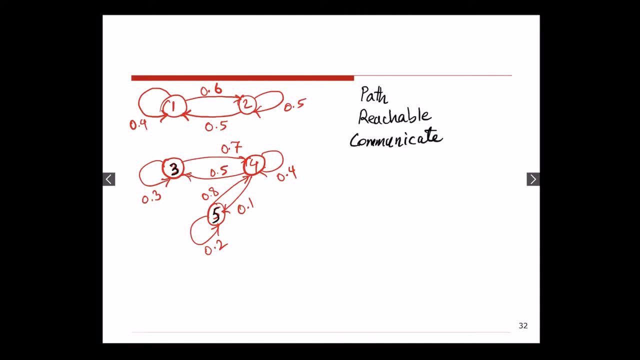 5 form a closed set. What does that mean? It means that state 1 and 2 are not reachable from any other state. State 3, 4, 5.. State 3, 4, 5, form another closed set. That means these three states are not reachable from any other state. 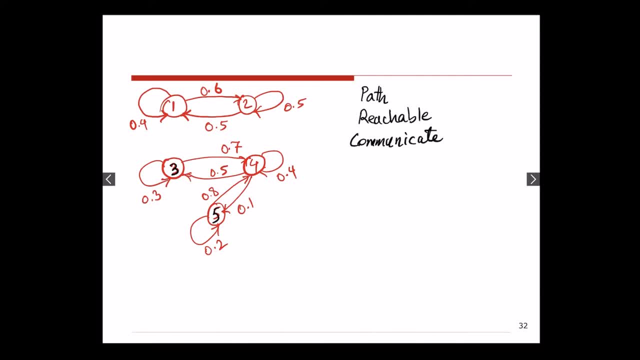 State 1 and 2.. Okay, So in this scenario, state 1 and 2 form one closed set, and then state 3,, 4,, 5 form another closed sets. Okay, And then The next definition is the definition of absorbing chain. 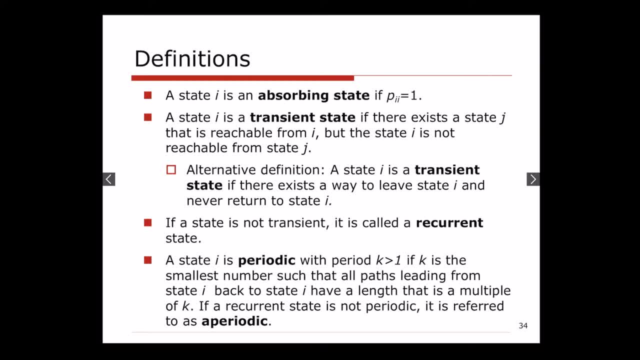 Absolutely Absorbing a state. So if for each state I we have the probability of transition back to the state I equals to 1. We call that an absorbing state. So if I want to give you an example, if you remember, 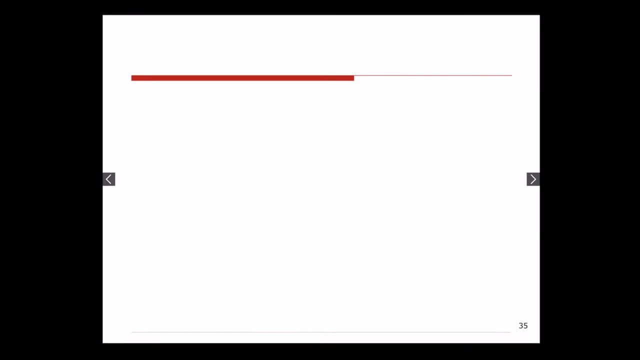 in the gambling example than we had with. the person had $2 and the person was going to play the game. in each hand he was going to gain one dollar or lose one dollar, till the person loses everything or gains four dollars, and then that person would quit the game. so the possible states for the 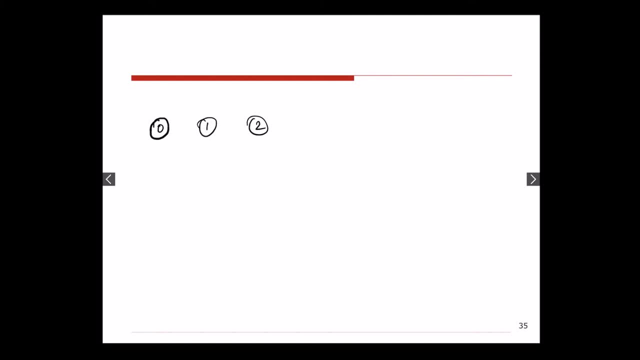 person were zero, one, two, three and four, if you remember. if the person would get to zero dollar, the person will quit the game. so the this is the state that we always will stay in. if the person will get to the four dollars, the person would quit the game as well. so this is the only state. 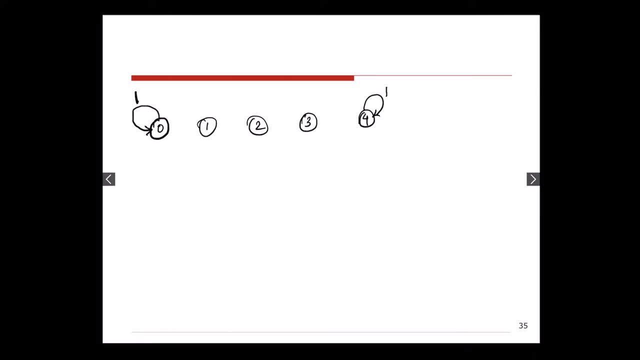 that we would stay in and then if the person has one dollar, we may get to zero dollar. if the person loses the game with probability of one minus p, or if we win the game with probability of p, we will get to the two dollar state. similarly, for the two dollar if we lose we get to one, if we win, we get. 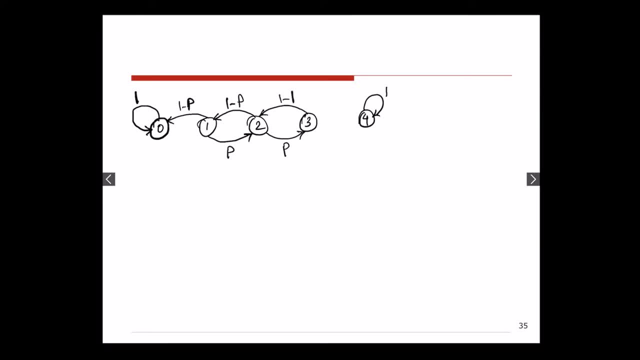 to the three dollar. if we lose, we get to two dollar. if we lose, we get to three dollar. if we lose, we get to two dollar. if we win, we get to the three dollar. win, we get to four dollars. okay, obviously i cannot go from four to three, because when we 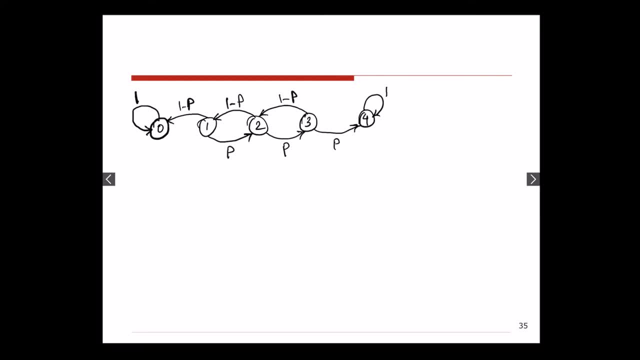 get at the state four, we quit. i cannot go from a state zero to one because when we get to zero we lose the game and we quit as well. so this is the state diagram for this, for the gambling problem. so, if you remember the, the last definition that we looked at was definition of absorbing a state. 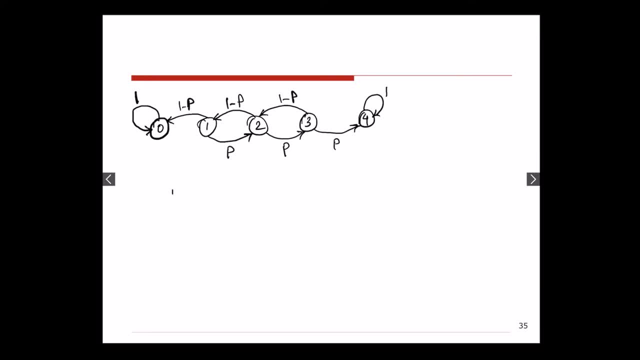 we said that if for a specific state, for example state zero, probability of going from state zero to state zero is one, we call that an absorbing state. okay, this also holds for state four, because you know, if you are at state four, probability of staying at the state four is one, so we call those. 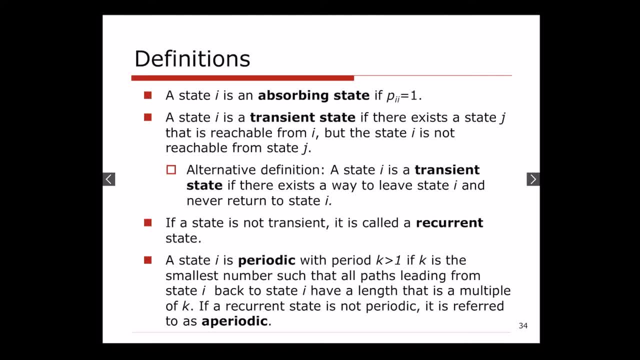 states absorbing states. the other definition that we have is the definition of transient state. so let's see what is transient states. if there is a path for each state i, we call that state transient. if there is a path that can take us from state i out and never let us to go back, 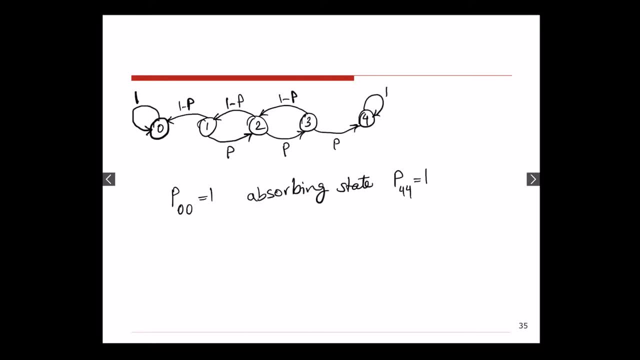 then that's the scenario. we call that state a transient state. so let's look at this example again. if we consider state two, for example, obviously there there is a path here that can take us from state two. for example, i can go to state three, but i can also come back to state. 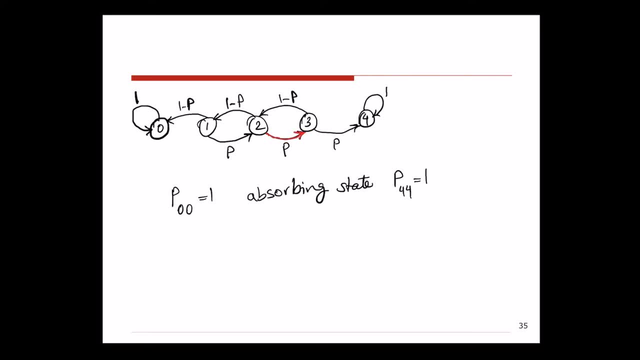 two. okay. so this is a path that can take me out of two, but also it will lead me to two as well. another path that can take me out of two is this one: i can go to one, but i can then come back to state two as well, okay, however, there is at least one path that can take me out of state two, and i 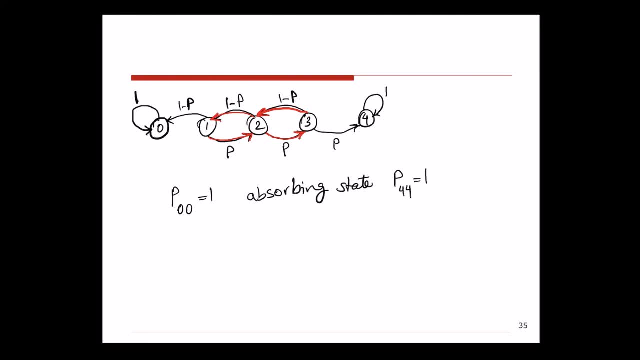 and never let me to go back. so, for example, if i go from state two to three and then i go from state three to four, then i would end up staying at the state four forever. so there is at least one path here, this one that takes me from state two to state four and never let me to go back to state. 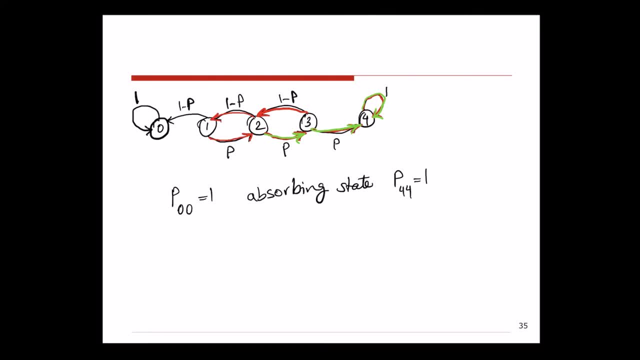 two. in that scenario, we call a state two a transient state. if you look at this model, uh, this uh stochastic process, we will see that this is the same case for state three. there are paths that that that can take us out of state three, but let us go back and there is at least. 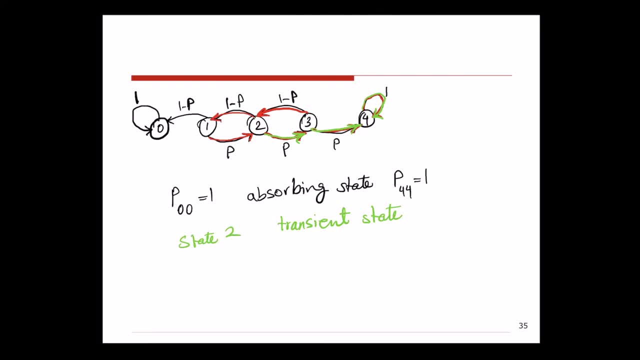 one path that can take me out of state three and never let me go back, and that's the the path that takes me to state four. um, similarly, there is a path that can take you, for example, out of state three and that can take you to say zero. so, for example, if i go through this path, 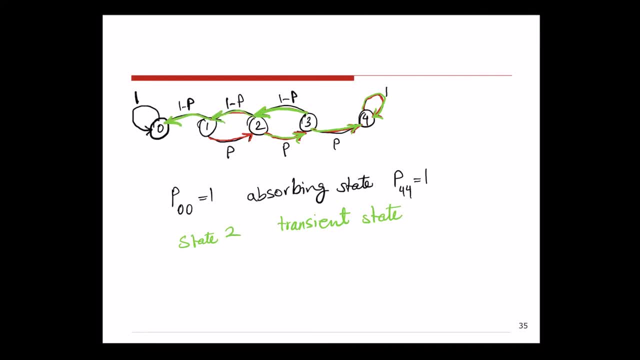 and then this path, and then this path. I will end up staying at the state 0 forever. So there is at least one path that can take us from state 3, and it doesn't let us to go back again. So state 3 is a transient state as well. 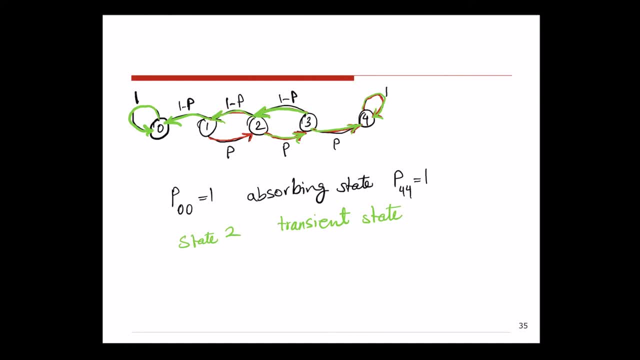 Similarly for state 1,, there is at least one path that can take us from out of this state and never let us to go back. So state 1,, 2,, 3, these are transient states in the systems. State 1, sorry. state 0. and state 4, those are absorbing states. 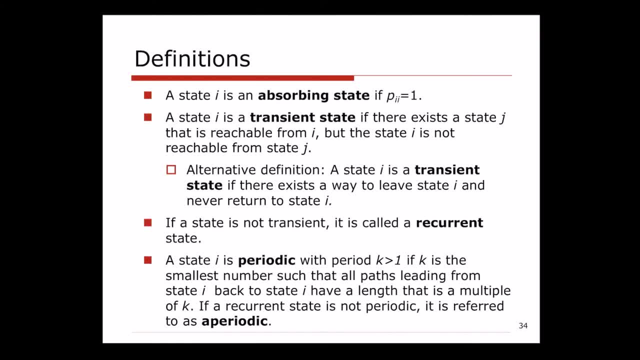 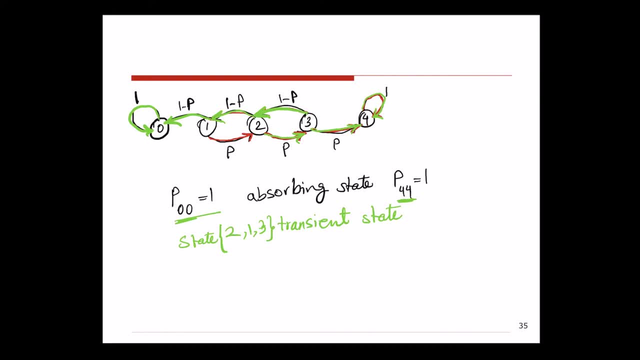 If a state is not transient, we call that state recurrent. So for example here state 0 and 4 are not transient states. They are absorbing, they are not transient. We call those states recurrent. Okay, So by however, pay attention. 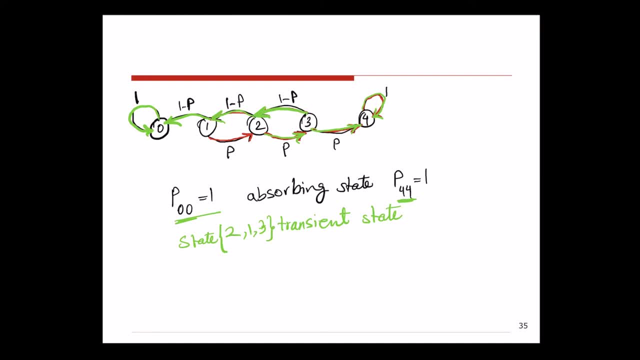 That absorbing states obviously, naturally, are recurrent, because once we get there we will stay there forever, So they reoccur again and again and again. But that doesn't mean that all the recurrent states are absorbing states. That's not the case. So, basically, if we have a state for which we cannot find a path that can take us out, 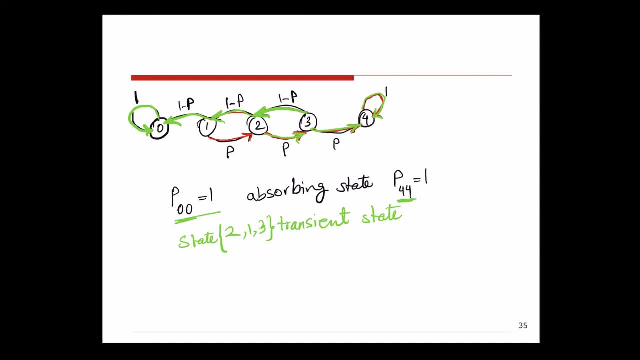 of that state and never let us go back. that state is recurrent. That means we can't go back. So when we leave that state, we always, always, always have the chance of going back to that state. Let me explain the definition of a recurrent state with an example better. 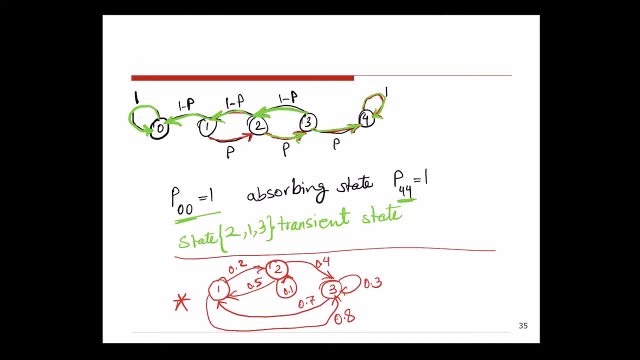 So in this example, let's assume we have three states. So in this state, as you can see, if we leave any one of the states- state 1 or state 2 or state 3, there's always a path that can bring us back. 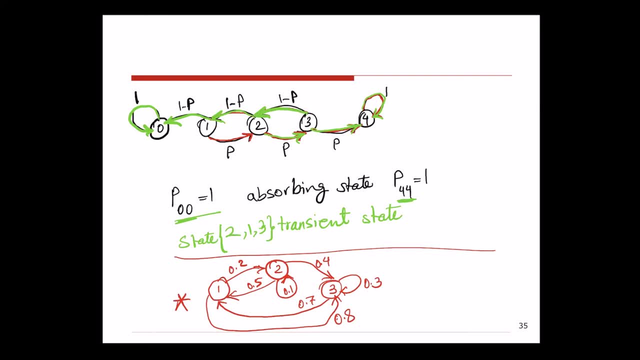 Okay. So you cannot find any path out of these states That would not let you to go back to these states. So in this example, all these states- state 1, state 2, state 3- are recurrent. Just pay attention that example 3 has a self-transition. 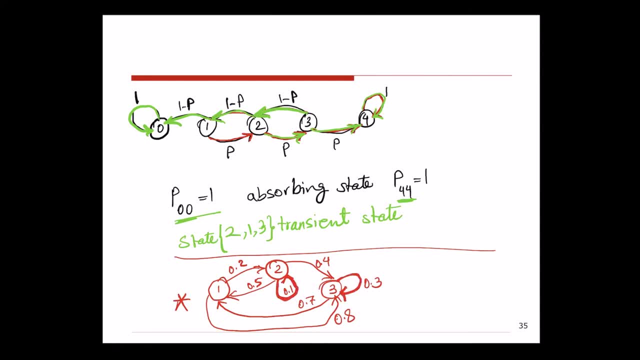 State 2 has a self-transition. However, these self-transitions do not happen with probability of 1.. They happen with probability of less than 1, 0.3,, 0.1, and so forth. So only if a self-transition happens with probability of 1,. 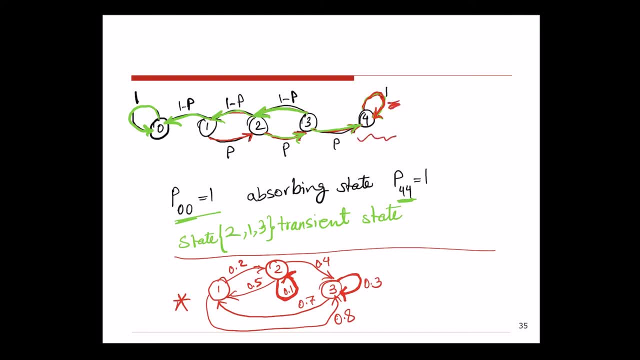 like the gamma is less than 1,, 0.3,, 0.1, and so forth, And like the gambling example, that's when we call it absorbing a state, But other self-transitions that happen with a probability of less than 1,. 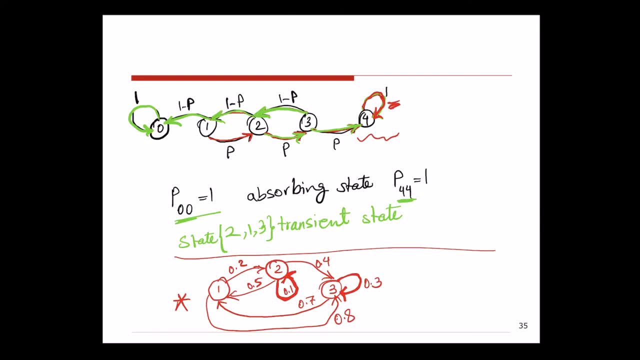 that means that if you are at state 3, sometimes you may end up staying in this state in the next time step, or you may end up going to state 1 with probability of 0.7.. Okay, So state 3 is not absorbing a state just because they have a self-transition. 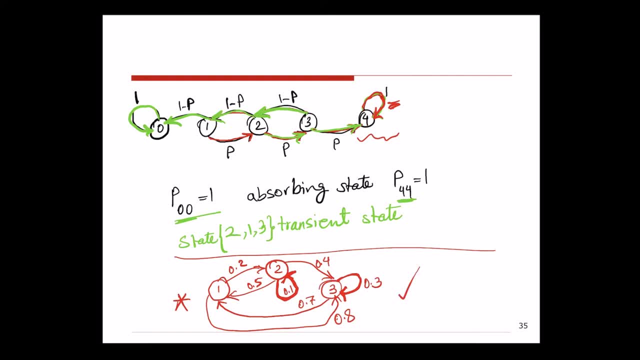 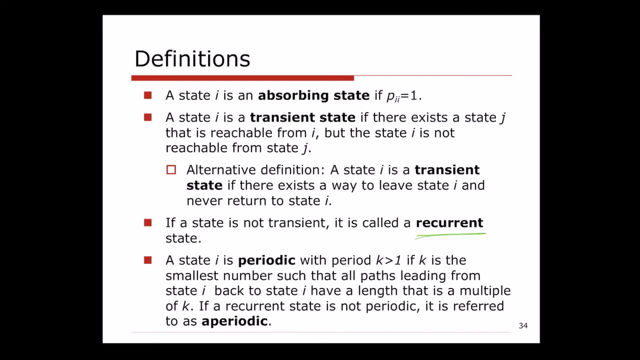 So in this example, all the states are recurrent and, as you can see, they are not necessarily absorbing. State 1, state 2, state 3 are recurrent, And then, lastly, I want to define the periodic definition for this state. 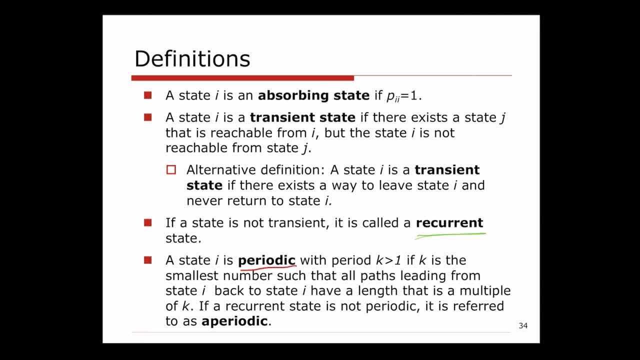 So for any state- i we call that state periodic- If we find the length of the shortest path that can take us out of that state and let us go back. and every other path that is taking us out of that state and letting us to go back has a length that is. 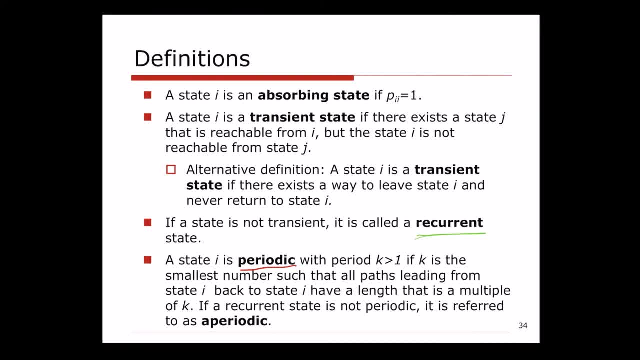 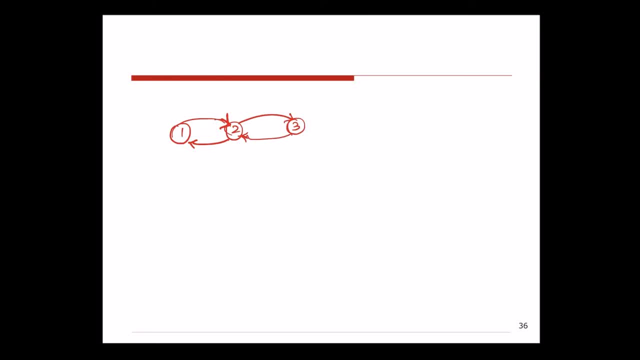 among other things, less than 1,, 0.3,, 0.1, and so forth. So that's the multiplication of that shortest path. Okay, So let's look at another example here. So in this example, what is the length of the shortest path that can take us from out of state 1? 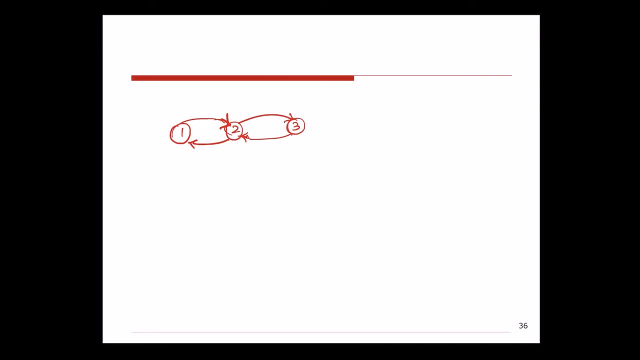 and then bring us back to state 1?. So the length of that path is 2, right, Because there is 2 transitions. I can go from 1 to 2 and then 2 to 1.. Okay, What is the length of other paths that can take me out of 1 and let me to go back to 1?? 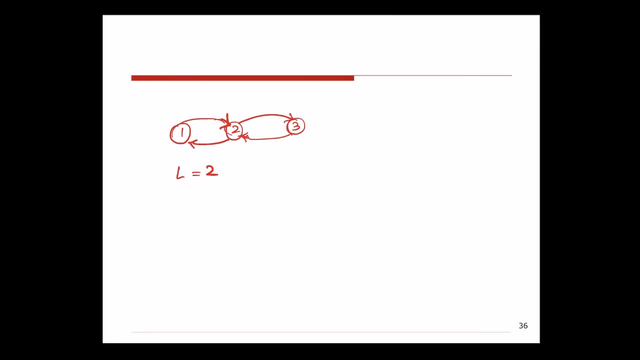 So the other path. we'll be going from state 1 to 2,, 2 to 3, 3 to 2, and then 2 to 1, right, What is the length of this path? The length of this path is 4.. 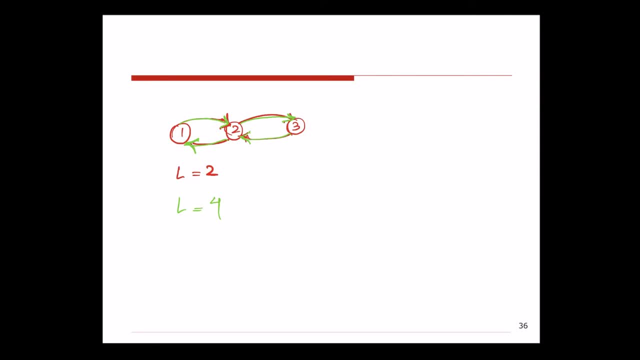 Okay, So we call state 1 a periodic state if the length of all possible paths that can take me out of 1- and let me to go back to 1, is a multiplication of the length of the shortest path that can take me out of 1. 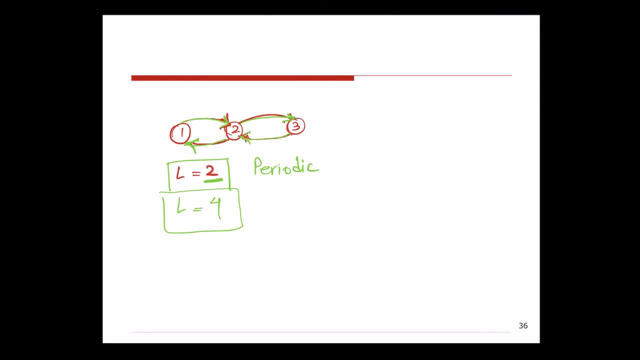 and let me to go back to 1.. Just pay attention that the length of this shortest path- for example, I call it k, the length of the shortest path that is taking me out of state i and bring back to state i, should be anything greater than 1.. 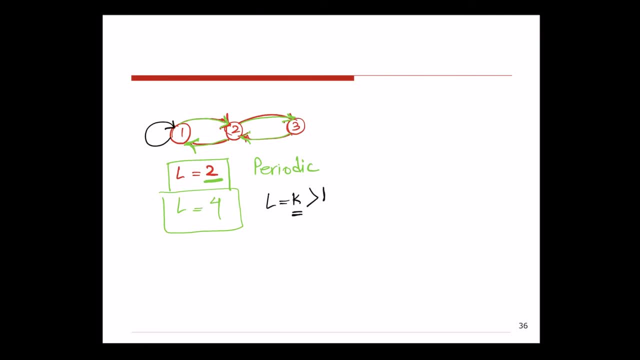 Okay, So if I have a self-transition here, that's not considered as a periodic state, So that definitely should be excluded. So I, if I count the length of the shortest path that take me out of state 1 and bring me back to the state 1,. 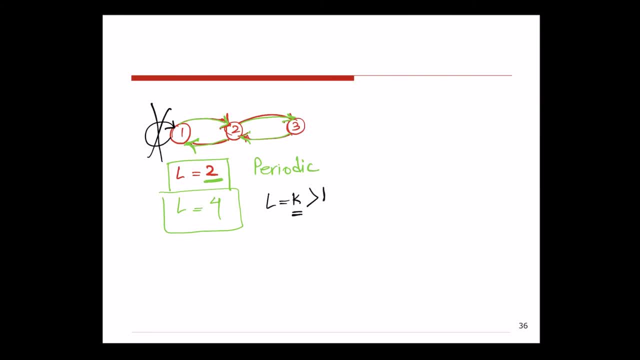 that definitely should be greater than 1.. And then if for any other path that takes me out of state 1 and back to state 1, if the length is a multiplication of the shortest path, we call that state in a periodic state. 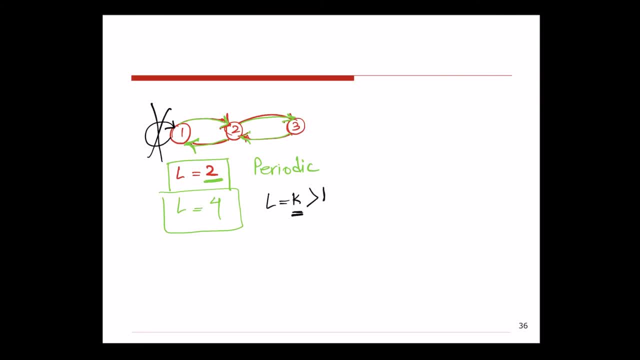 meaning that I can find state 1,, for example, in two transitions here, or in four transitions, and that's all. So it happens periodically in two or four times. There's a third answer to this question as to why you should look at a state. 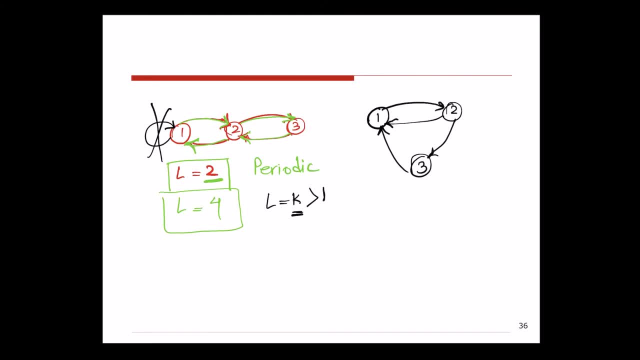 one逅 Goldruth graph and that a higher Looking for error is. see if the third answer, which you see in the bottom is, is really important. Okay, So if I, if for any other cohort, if you want to call it positive n. 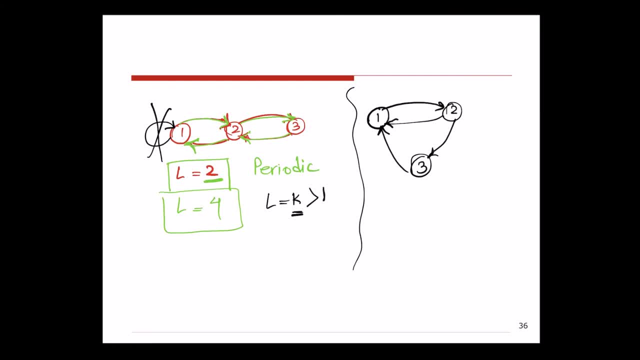 the second answer is: if you, if you have you say the number, then what is positive? And I put negative over from 0. Okay, Okay, Okay, Okay. So now you have the lessons part. These are the lessons students got. 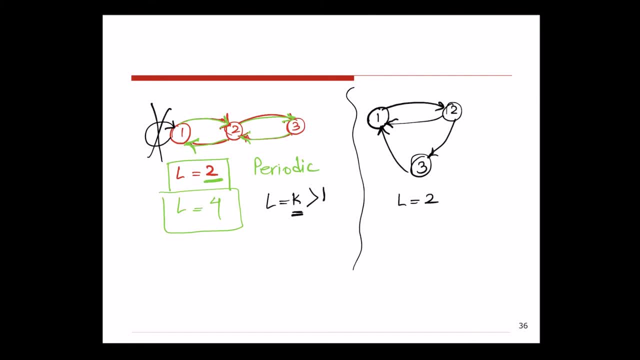 So these are lessons students will learn. So if you look at this example, this is the classic method. This example is 60 tech behavior. here There's n levels C in group b, only the other path that can take me out of state one and bring me back to state one the length of the. 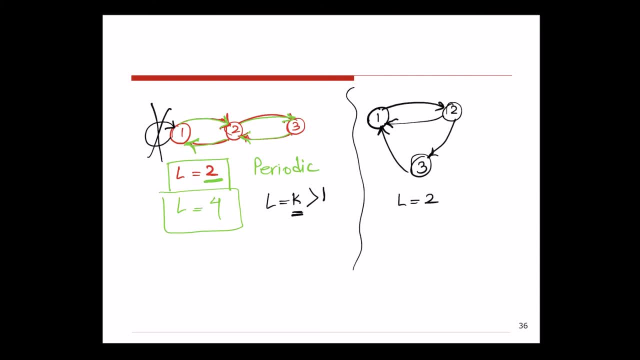 other path is going from one to two, two to three and then three to one. so the length of the other path is going to be three, three transitions and, as you can see here, um, state one is not periodic, so we call it state one is a a periodic state. it's not periodic. we call it a a periodic it's. 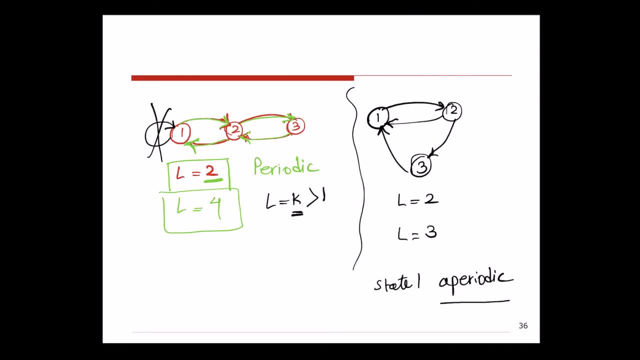 a periodic state because the length of the shortest path that i that can take you out of one and bring back is two. however, we found another path whose length is not a multiplication of the minimum length, which is two. we found another path out of state one and back to state one. 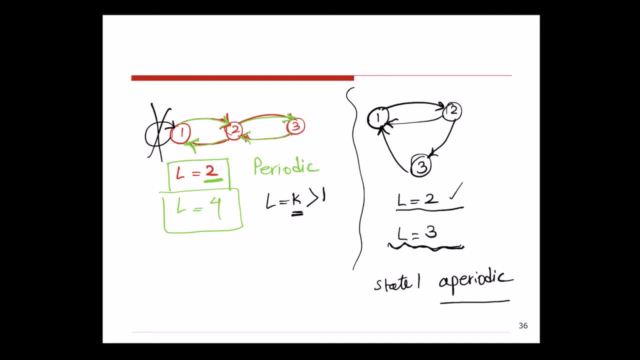 whose length is not a multiplication of two, which is the length of the shortest path from one out of one and two one. okay, so in that scenario we call the state one and a periodic state. usually when we look at the markov chain, um, all the states turn out to be a periodic or periodic. 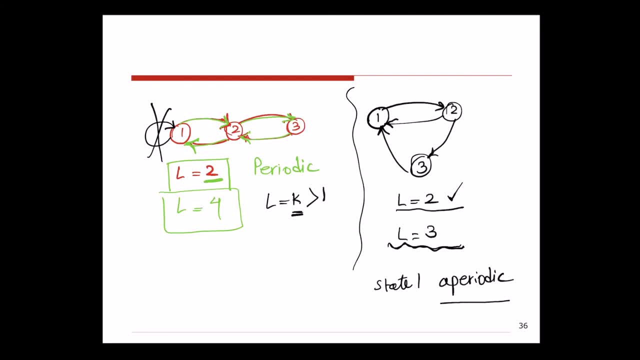 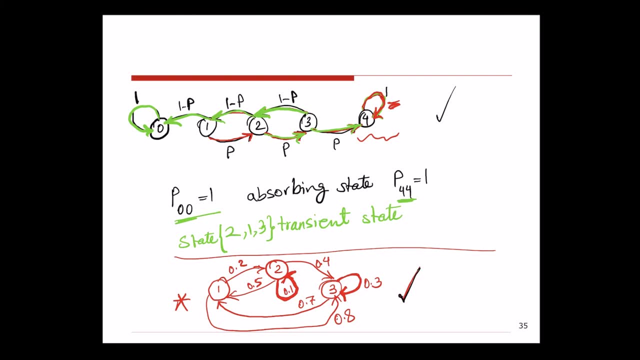 if you infine your um states, um, for example, similar to the gambling ones, or even in this example, in both these examples, whenever you have a self transition in your markov chain chain, that just immediately um removes the chance of um being a periodic state, because obviously the shortest path. 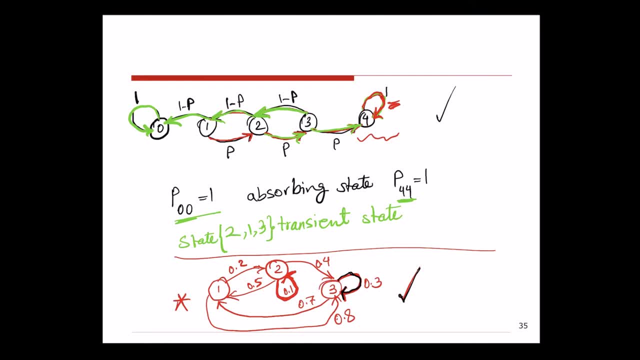 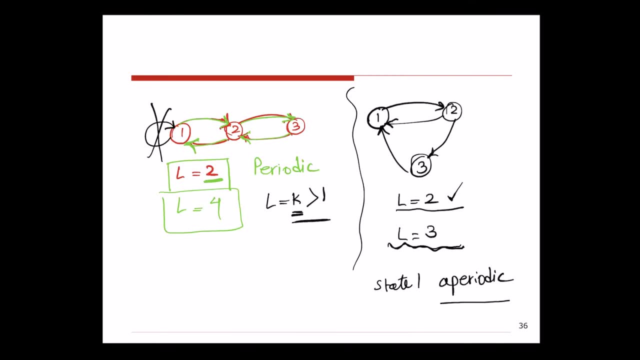 that can take you out of three and back to the tree, is one. but remember, in the definition of the periodic state we said the shortest path should have a length greater than one. so whenever you see a self transition from any one of the states back to itself, that immediately says that that state is not. 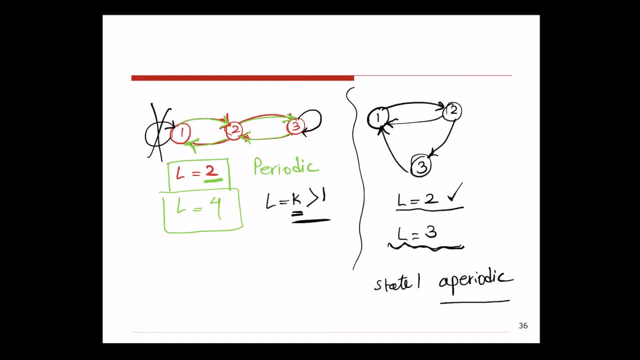 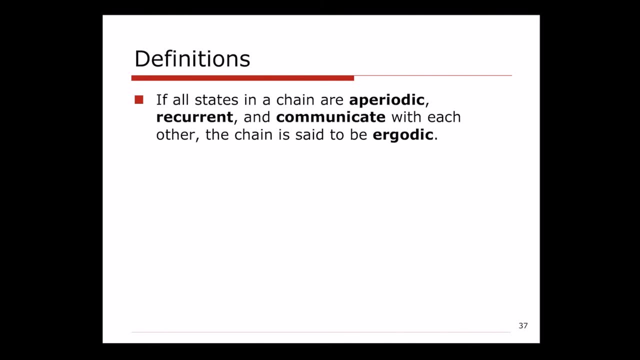 periodic and um and, as i say, usually in the mark of chains all the states end up to be periodic or a periodic. and lastly, if we have a markov chain in which all the states are a periodic, recurrent and communicate, we call that markov chain a periodic state and we call that markov chain a. 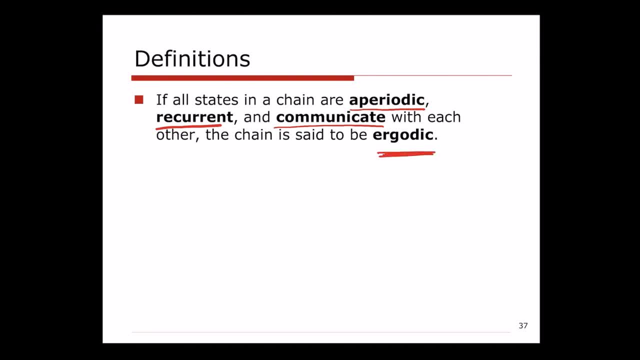 ergodic mark of chain. okay, this is important. uh, why do we need to know that? because when we are going to study the behavior of markov chains in the long term- um, in the in the long time- then we are going to look at ergodic mark of chains. so we have to make sure the mark of chain that 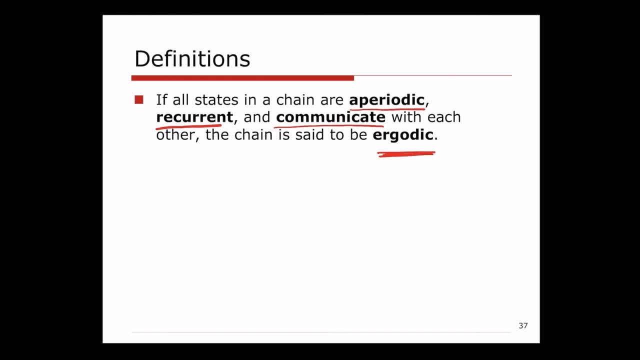 we are analyzing has these characteristics, before we can say anything about the long-term behavior of that mark of chain. okay, so, uh, let's look at one example, and so what i'm going to do is that i'm going to draw the state diagram of this transition. 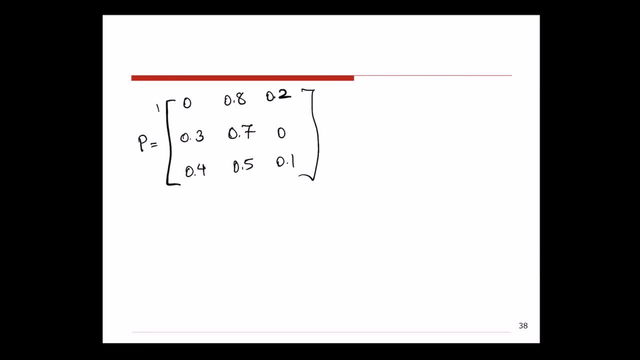 probability matrix and just note that we have three states: state one, state two, state three. okay, this, so this is the state diagram of. so now we want to check if this uh markov chain is ergodic or not. and remember, we have to have three things for a mark of chain to be ergodic. 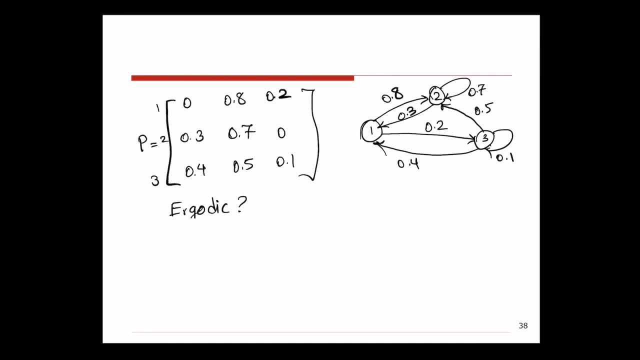 it should be recurrent- all the states should be recurrent, communicate and and also be a periodic. so let's check these um: a three characteristic in this mark of chain. what was the definition of recurrence? so in the recurrent states, we want the that states to happen always. so when we leave, that states we don't want. 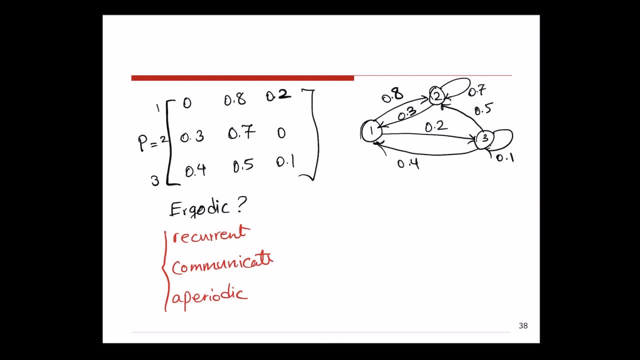 to have any path that can take us out of that one state and never let us to go back. if we look at here, we cannot, for any one of these states, state one, two, three. we cannot find any path that can take us out of that state and doesn't let us to go back. so all these states are recurrent for sure. how? 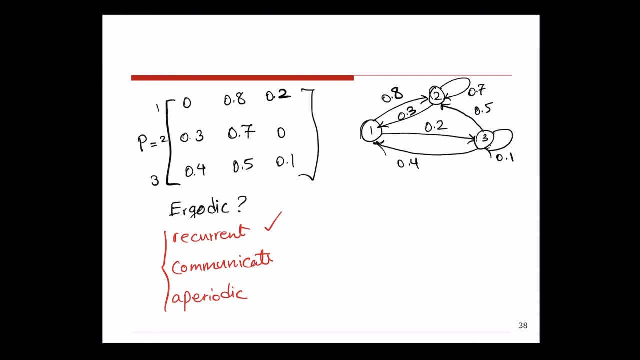 uh is so communicate, for between every two state means that there is a path from state i to j and there is a path from j to i. so obviously we can go from state one to two, two to one, one, two, three, three to one and then two to three and three, two, two. so for example, i can go from state two to three. 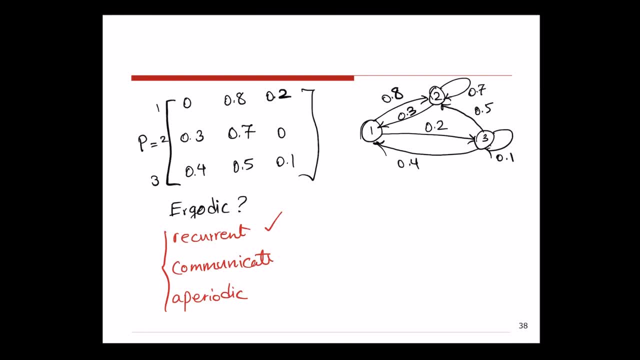 by going from two to one and then one to two. when we say there is a for the communicate, communicate a scenario when we say there is a path from state i to j and j2i- remember this can be a path of multiple transitions, it shouldn't be just one transition. 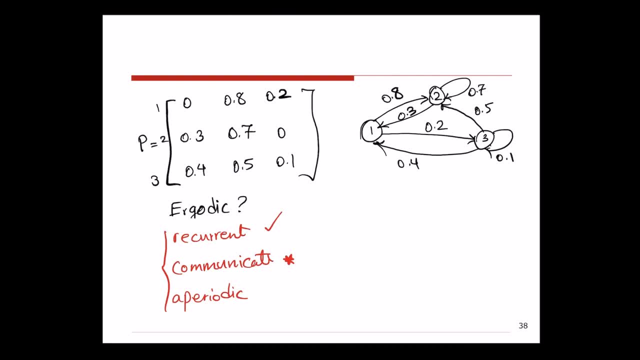 so, for example, as i said, from state two to three, we don't have just one transition that take us directly from two to three. but that's okay. as long as we can find a path that that can take us from two to three, we are good. we can go from two to one and then one to three, so state three is reachable. 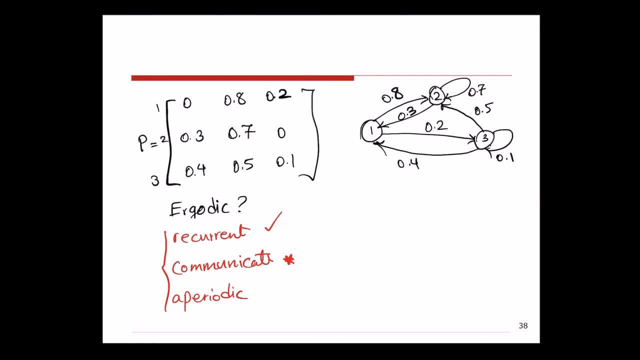 from two, and that's that that works. so all these states communicate as well, and then, uh, we need to see if they are aperiodic or not. as i said, as long as, as soon as we see a self-transition, that definitely, um, opposes the definition of being a being periodic states. so because now the length? 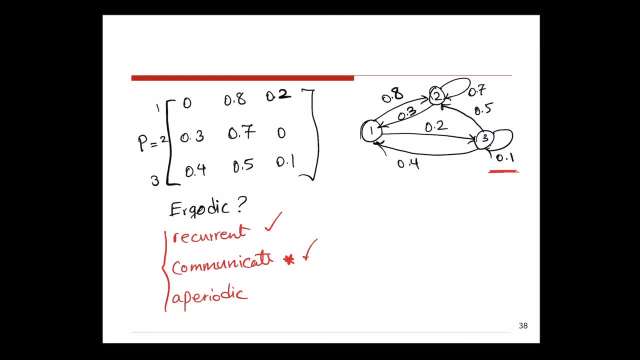 of um shortest path that can go from three to three, is one instead of a number greater than one. the same so for the two, and so we don't in this. uh, in the definition of ergodic um markov chain, we need to have all the states aperiodic, which is the case here. none of the states are periodic in